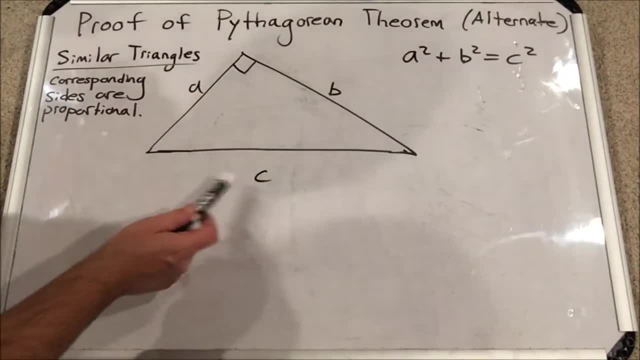 angle is equal to the square of the hypotenuse for a right triangle, that's the side opposite the right angle. Those of you who've done geometry at all, you're very familiar- maybe even algebra- with this formula. Now, this proof makes use of a right triangle specifically. 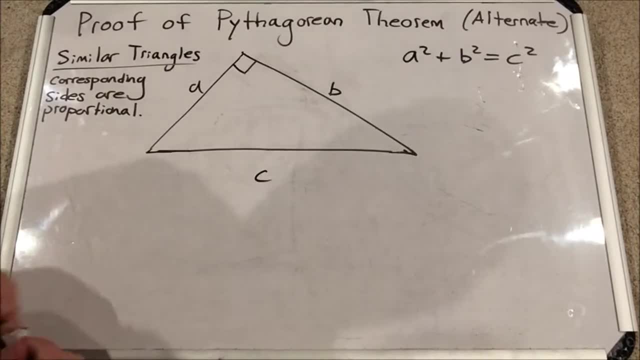 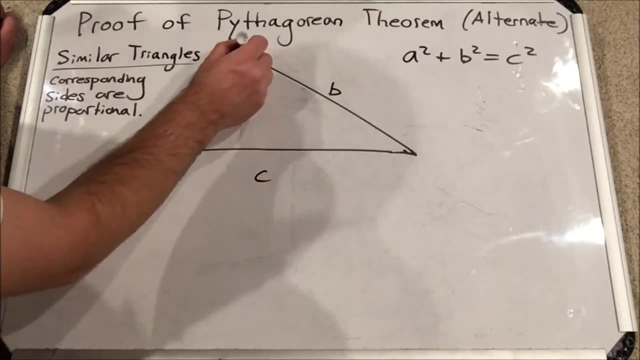 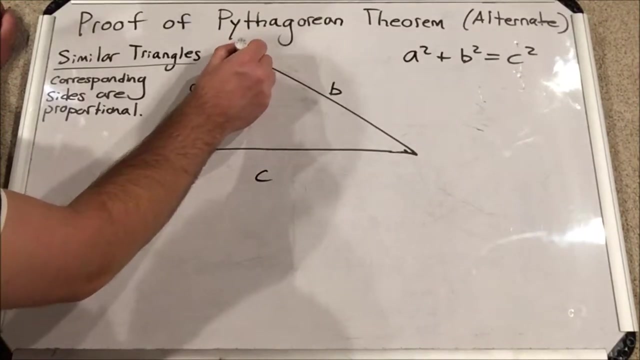 and I've labeled the sides as such: A, B and C. Now what you do for this triangle is you make the altitude from the hypotenuse. So I put the triangle on its side, such that the hypotenuse is at the bottom, and I make an altitude which is a line that is perpendicular to one of the sides. 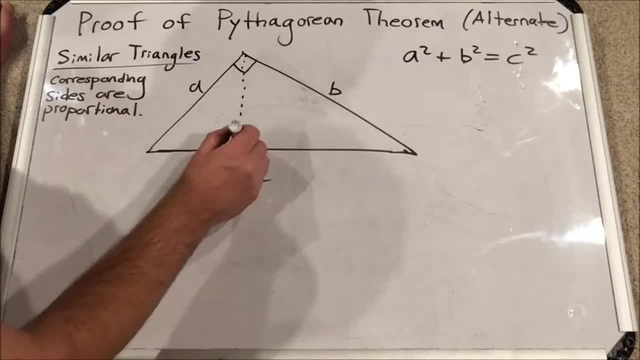 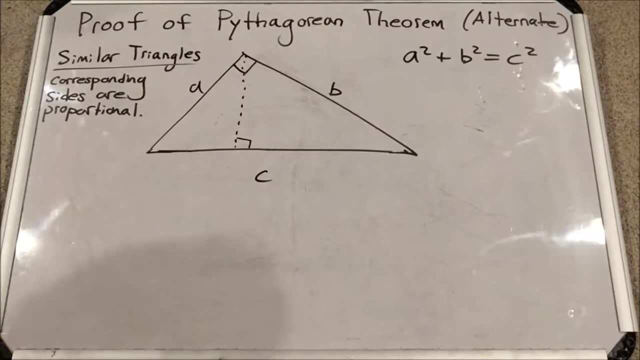 and extends to the vertex of the opposite angle. So this is a right angle here as well. I'm going to label the sections of side C that are cut by this altitude right here. I'm going to label the short part here: Z. So this section, I'll move this down. this section right here is Z. 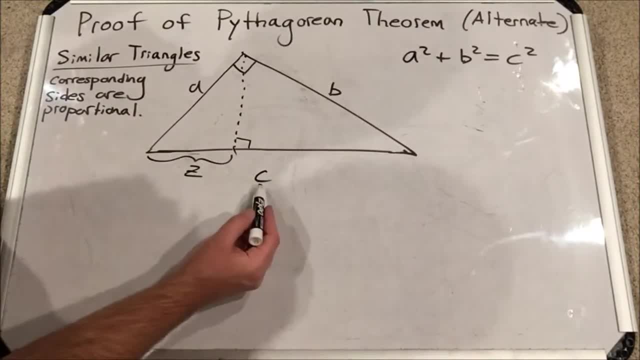 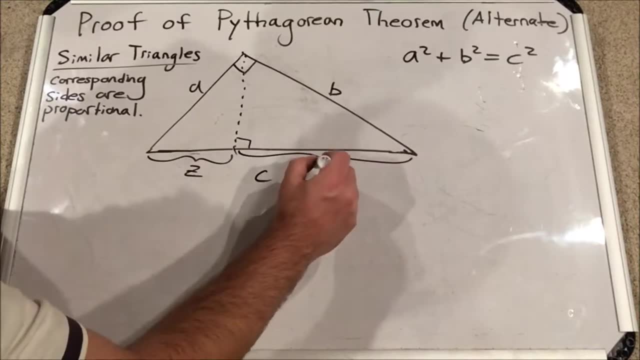 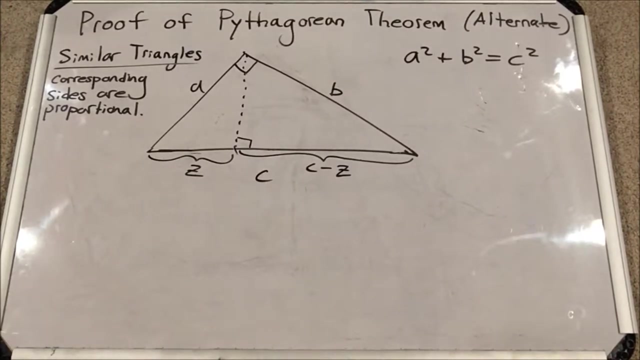 Then over here, this would be the leftovers of C. So I'd subtract Z from all of C and I'd get this portion. I'm literally going to label that C minus Z. So now that I have that labeled, I'm going to make use of the fact that I've created three. 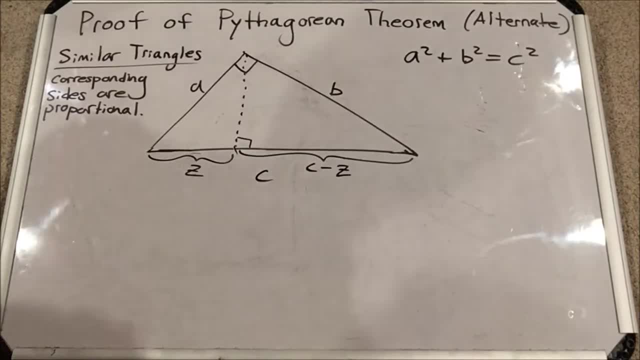 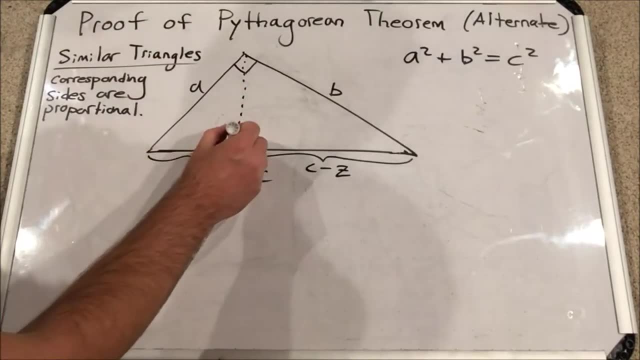 similar right triangles out of one. And this is what you do when you make the altitude from the hypotenuse to the right angle, You actually make three similar right triangles. Now you have to remember what similar triangles mean. These mean triangles with the same angles, but proportional. 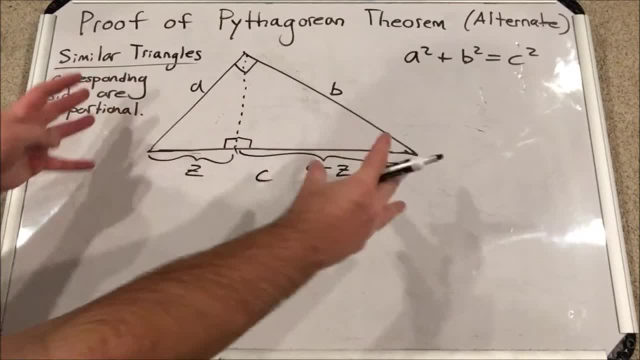 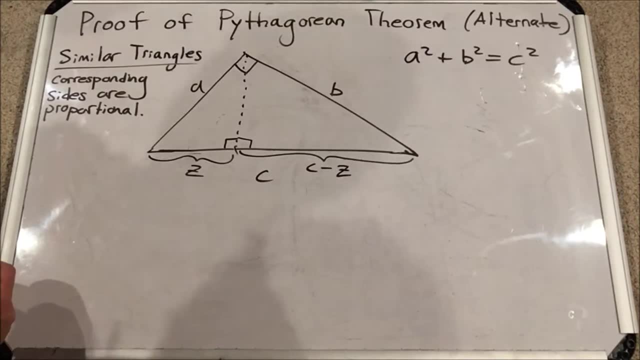 sides. So it's like I took one triangle or one shape and dilated it. So you have a certain scale factor, as you remember from if you've done transformations. yet There's something true about similar triangles that have the same angles and proportional sides. 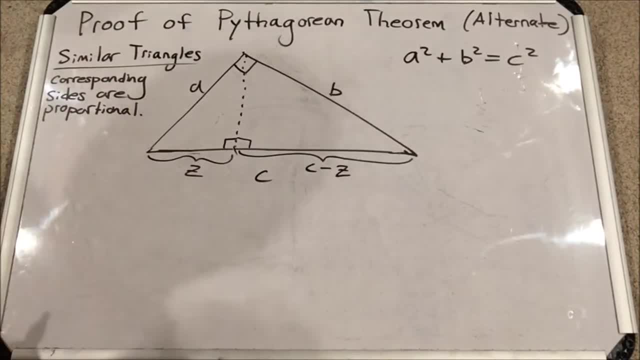 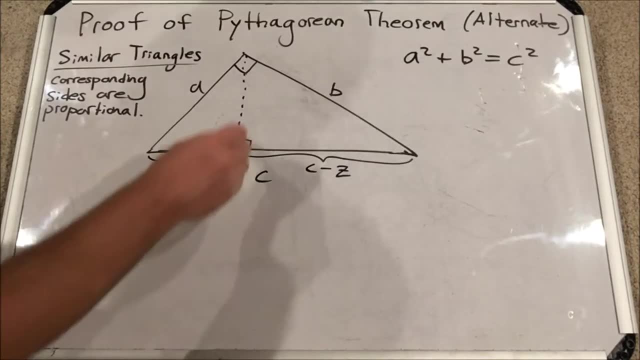 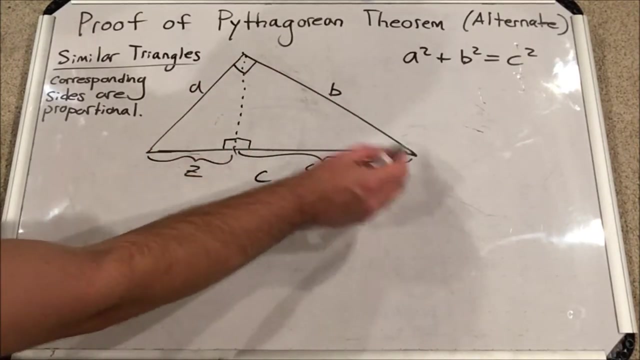 Well, just that. that is true. Corresponding sides are proportional. That means I could set up proportions of corresponding sides, And that's what I'm going to do here. So this triangle here is the smallest of the three. This triangle here is the middle sized triangle, And then the main. 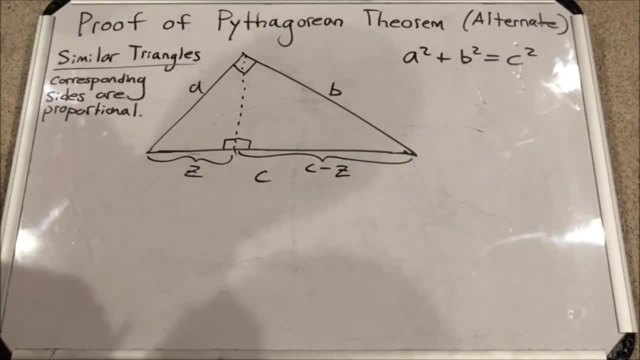 triangle is the largest right triangle. All three of those are similar to each other. I'm not going into that proof, but I'm assuming that's true for this proof. Okay, so now I'm going to set up some sides Now. I did not label the altitude because it's not involved in any of my proportions. 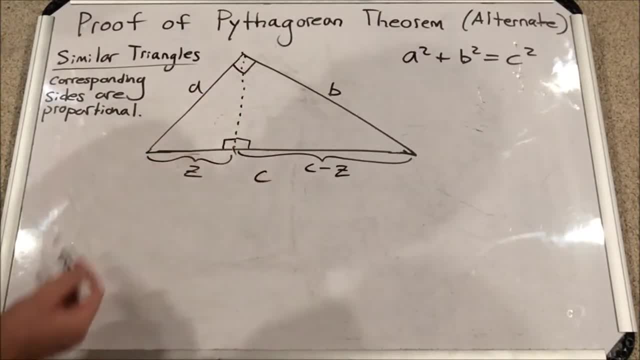 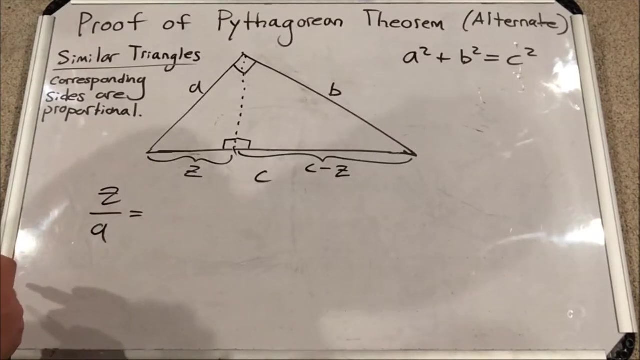 I'm going to look at the small triangle first, this one. here I'm going to take the shorter leg and the hypotenuse. I'm going to make a ratio of those two sides. Okay, now I'm going to look at and set that ratio equal to that same ratio of sides in the large. 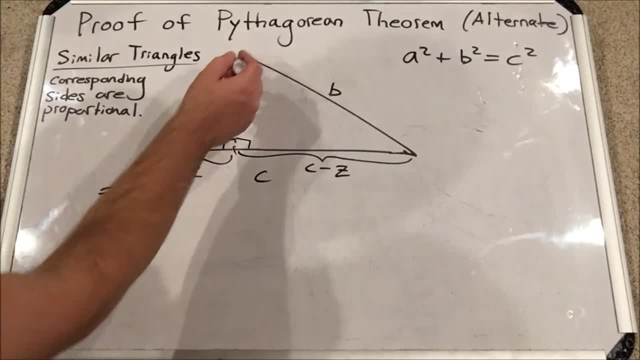 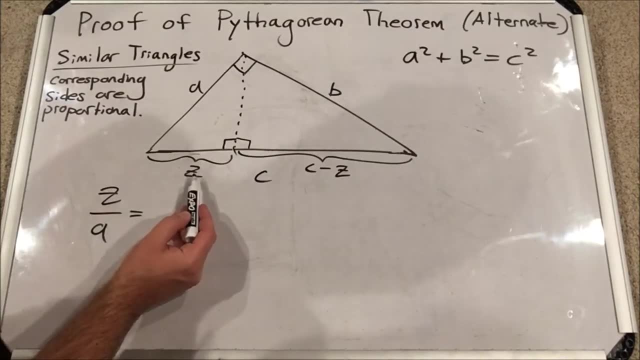 triangle. Okay, that would be. the short leg would be A for the big triangle and the hypotenuse would be C. So for the small triangle it was short leg Z over hypotenuse A, And then the large triangle. that's short side A over hypotenuse C. Okay, 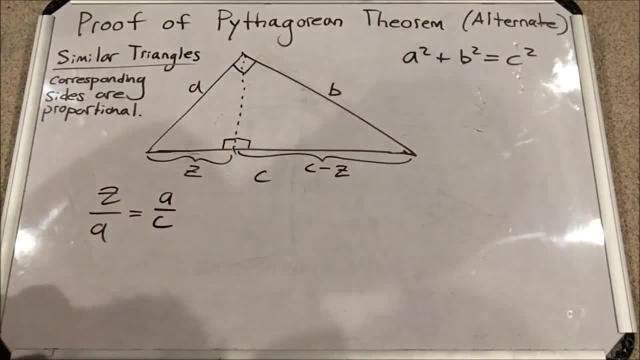 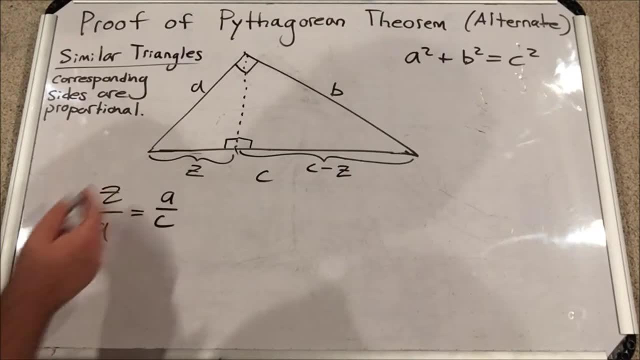 So Z over A would equal A over C. This is what some people refer to as baby equals mama type proportion. We've got the small sides in a ratio of the smaller figure on one side and the larger sides of the larger figure on the other side of your proportion. This is one proportion we're 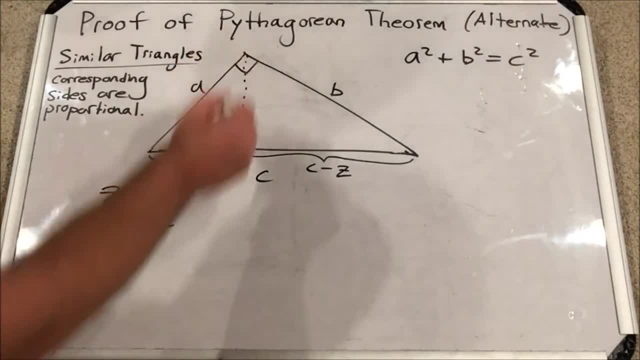 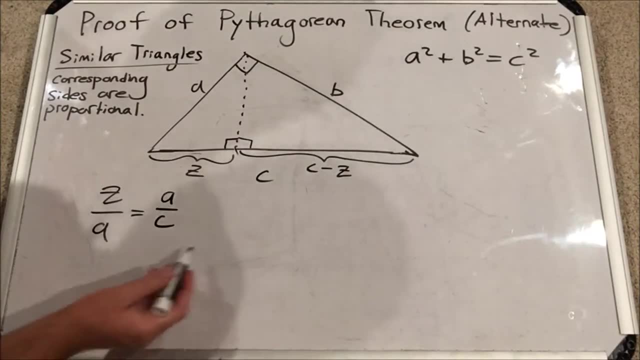 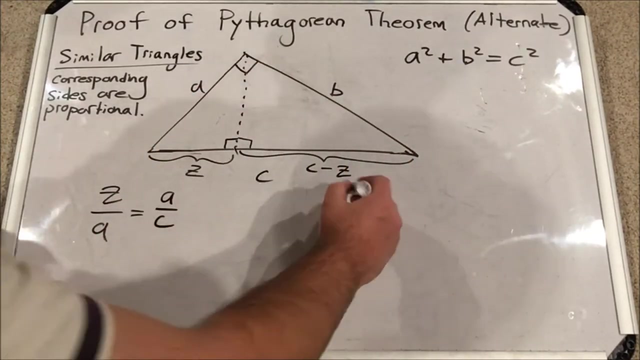 going to use Now. the other proportion involves the middle sized triangle and the large triangle. Okay, I'm going to do the same thing here, but with the larger leg. I'm going to set up a ratio of the larger leg which is C minus Z over the hypotenuse B. 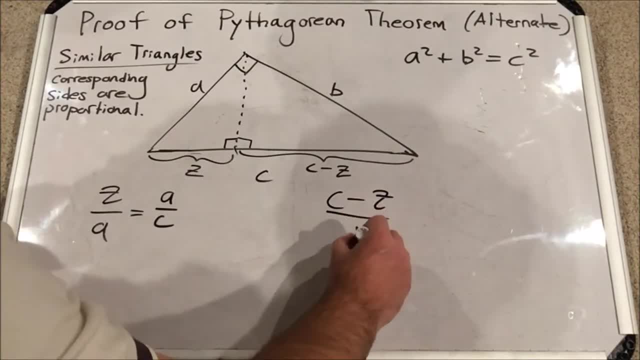 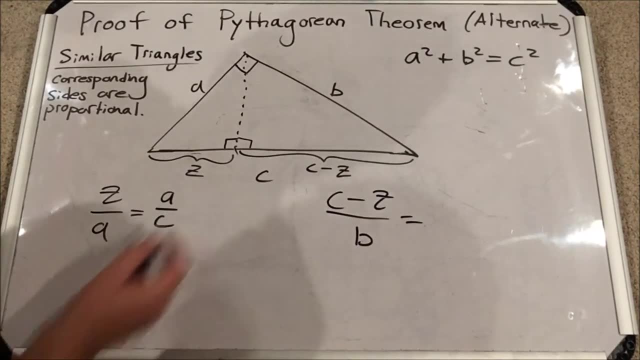 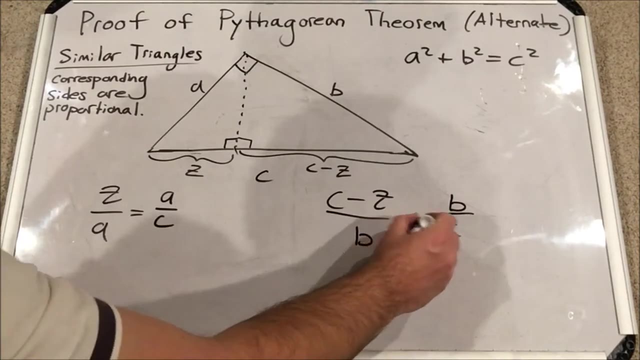 So I have C minus Z over B And I'm going to set that equal to the larger leg of the large triangle over its hypotenuse. That would be B over C, Like this. Okay, now that I have these proportions, I'm going to cross multiply. 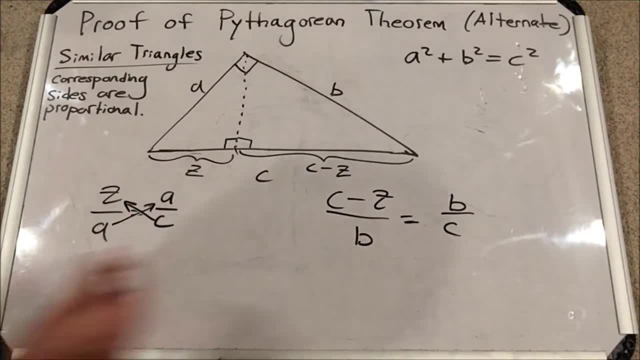 I'm going to multiply both sides by their respective denominators and so that these are no longer fractions, These denominators will move as the arrows point out. That's cross multiplication. That's one result you can get from cross multiplication Over here on this side. I'm going to get that A squared. when I multiply A times A equals C times Z.